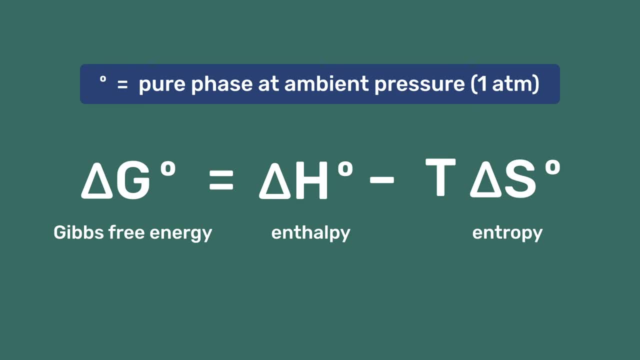 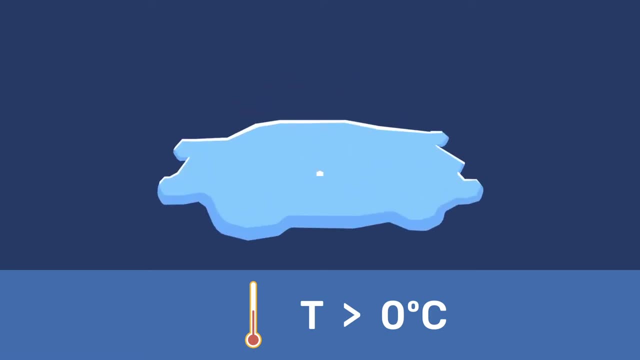 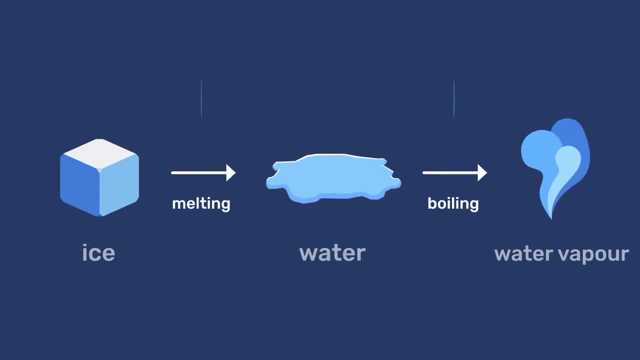 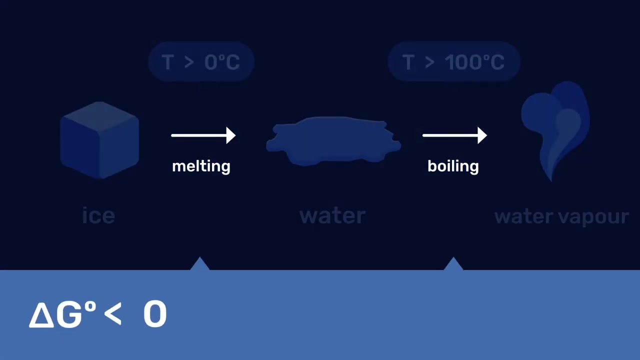 to indicate that we are considering pure phases. at ambient pressure Above 0°C ice melts and above 100°C water boils. Both processes are spontaneous in those temperature ranges. Their delta Gs are negative, But what are the signs of delta H and delta S for these transformations? Pause the video and think. 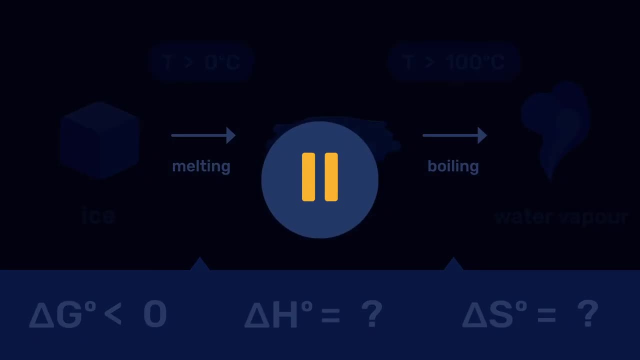 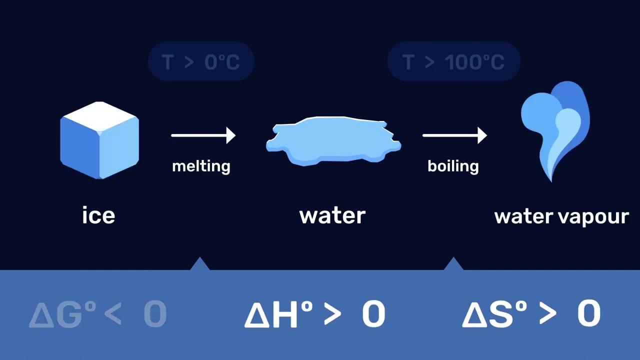 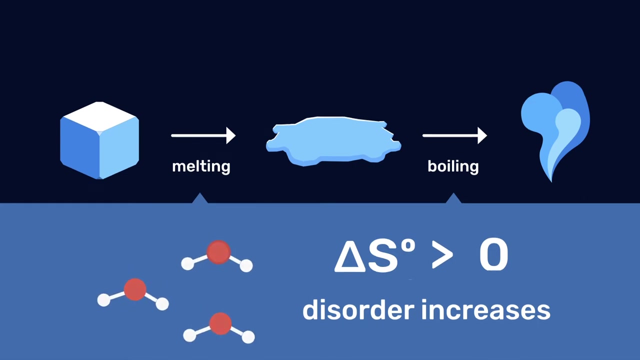 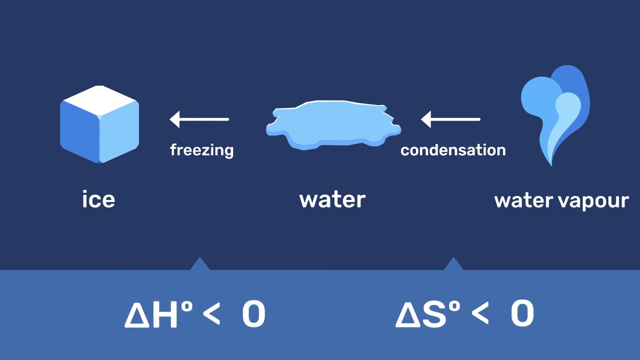 For the melting of ice, we have to consider the following transformations: For the melting of ice and the boiling of water, both delta H and delta S are positive because in both cases bonds must be broken and the disorder increases. If we consider the reverse reactions, both delta H and delta S are negative. 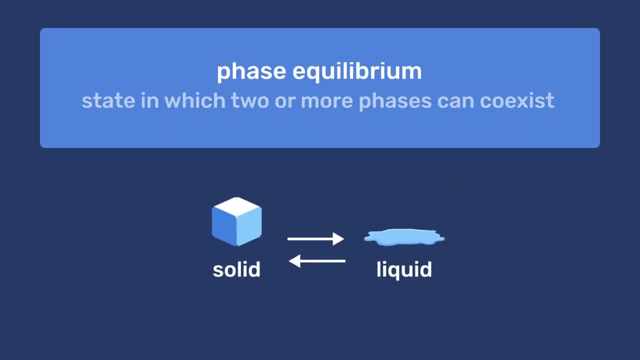 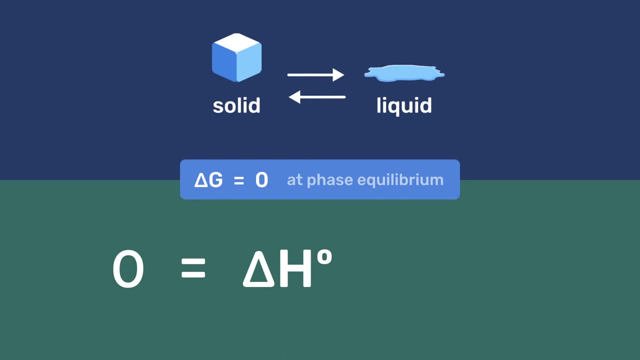 Let us move to considering phase equilibrium. This requires delta G to be equal to zero. This requires delta G to be equal to zero For the equation delta G equals delta H minus T delta S. we can define the melting temperature as: T melt equals delta H melt divided by delta S melt. 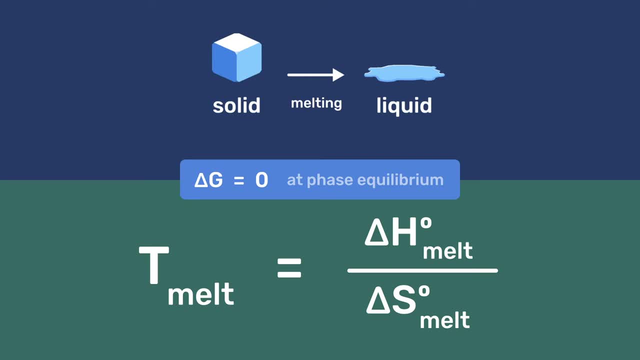 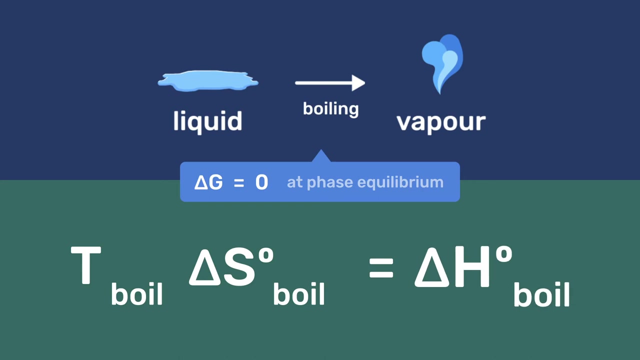 And we note that we get the same value if we consider the freezing reaction, since delta H freeze equals minus delta H melt, and that delta S freeze equals minus delta S melt. In a similar way, for boiling, we get T boil equals delta H boil. 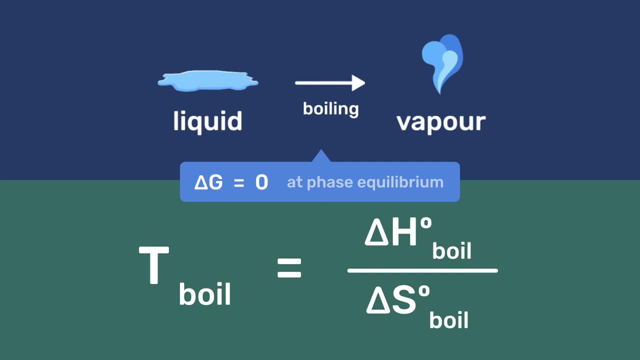 divided by delta S boil, the same value if we consider the condensating reaction, since delta H condensation equals minus delta H boil And T boiling equals T. deltah elits Aquatic condensation銖. Ur. multiple delta and ΔS condensates minus τhachen lake. 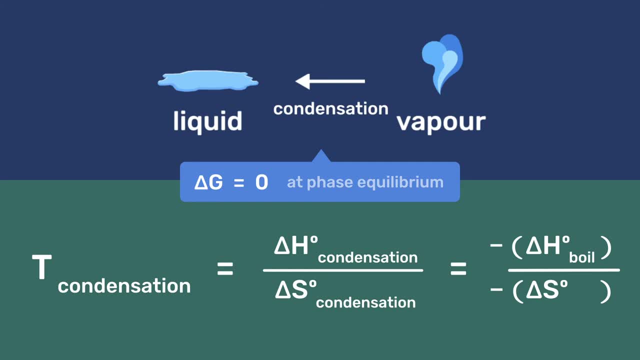 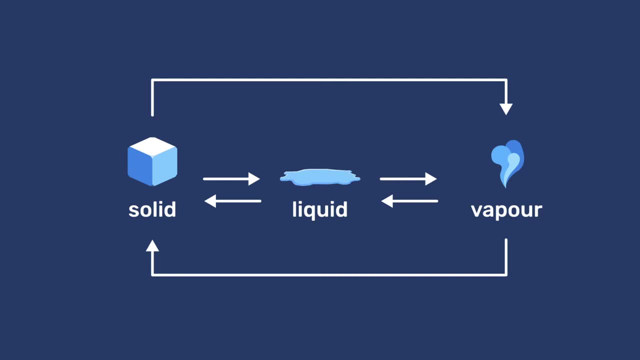 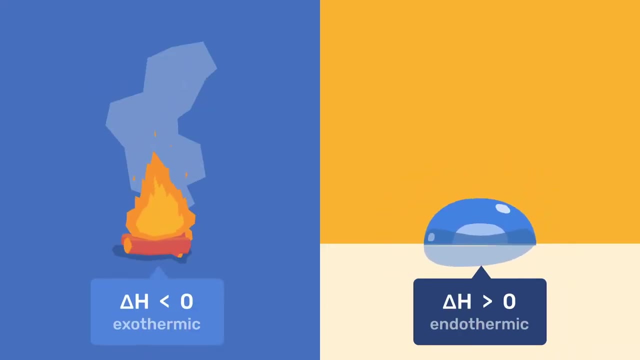 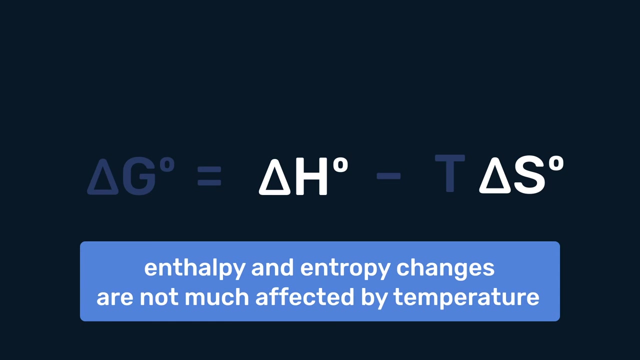 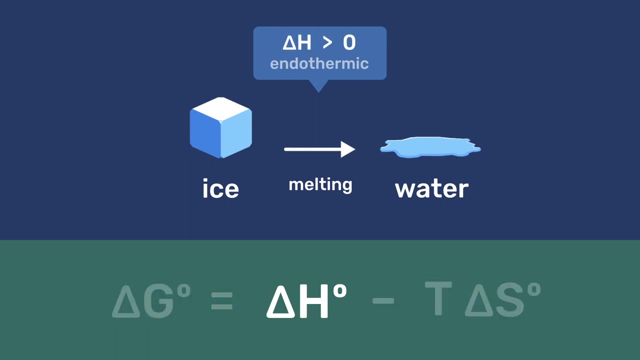 Fase changes are very important to understand the difference between spontaneous and non-spontaneous reactions, as well as between exo- and endothermic reactions. Enthalpy and entropy changes are not much affected by temperature, so the melting of ice is endothermic, with a positive delta H, regardless of temperature.